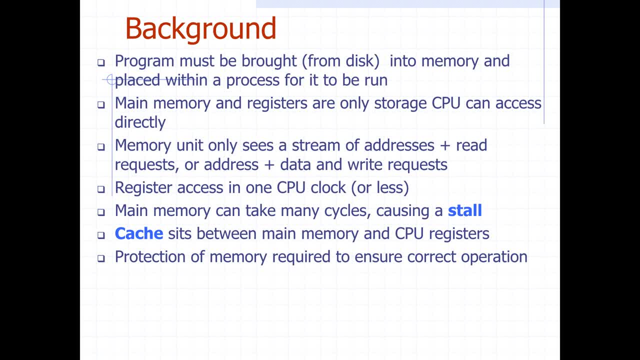 such as a disk into a memory or a main memory and must place within a process for it to be run. So again, a program must be brought from a disk into memory and placed within a process for it to be run. Now, main memory and memory management are two different things. 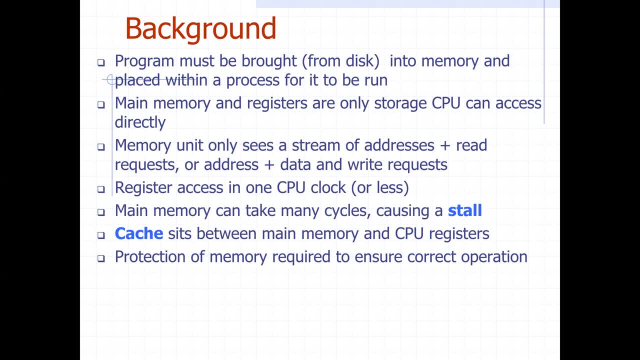 Main memory and registers are the only storage CPU can access. So, for example, a CPU cannot access a program or a file that is in a hard drive or is in a disk. It must be loaded into the main memory in order for a CPU to access it. 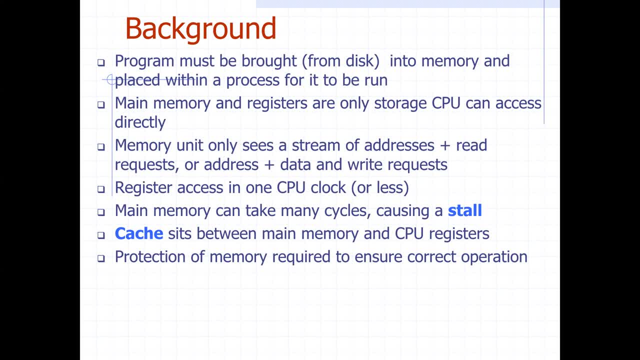 So memory unit only sees the stream of addresses plus read requests or address, plus memory. So it must be loaded into the main memory in order for a CPU to access it. So memory unit only sees the stream of addresses plus read requests or address, plus data and write requests. 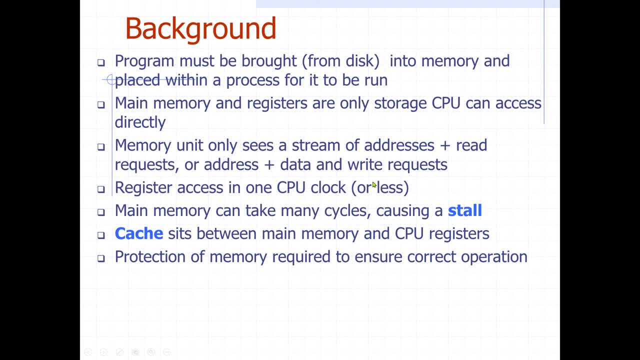 Also, we know the design of a memory management portion of an operating system depends on the three fundamental areas of choice: whether or not to use ventral memory techniques also, the use of paging or segmentation or both. Also, the algorithms employ for various aspects of memory management. 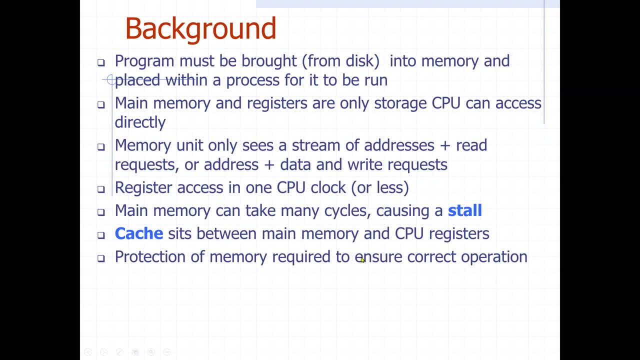 and we are going to cover some of the algorithms here. So again, a main memory can take many cycles, again causing a stall, And also caches sit between the main memory and the CPU registers, So the protection of memory required to ensure again a correct operation. 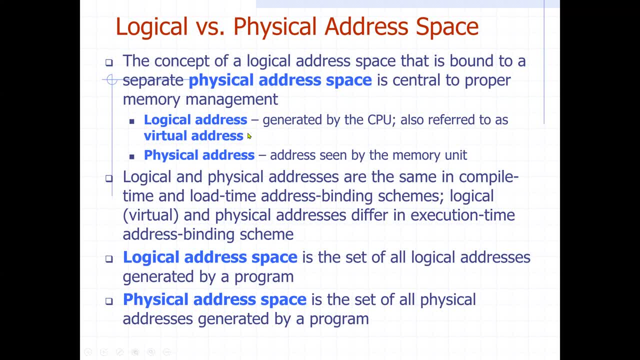 Here we talk about the logical and the physical address space. So again, the concept of a logical address space that is bound to a separate physical address space is essential to a proper memory management. So logical address normally generated by the CPU and is also referred to as a ventral address. 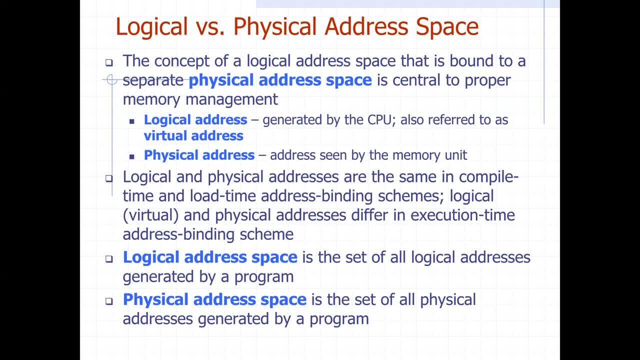 But a physical address is an address seen by the memory unit. So a physical address would be the actual address of the memory. Normally memory consists of cells, or we say a location, more or less like cells, that each cell have a unique address. 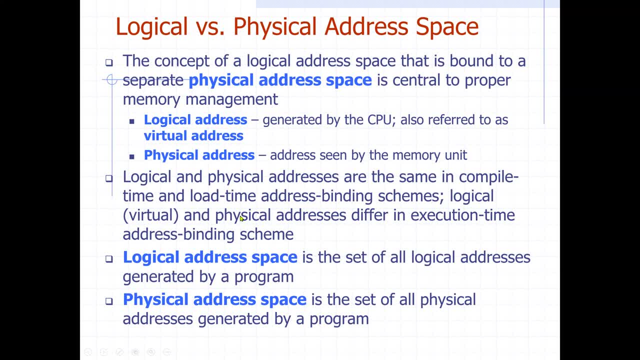 So again, the logical and physical addresses are the same in compile time and also the load time addressed by the schemes, And the logical or the ventral and the physical addresses differ during the execution time addressed by the scheme. So again, during the loading time, the logical and physical address are the same. 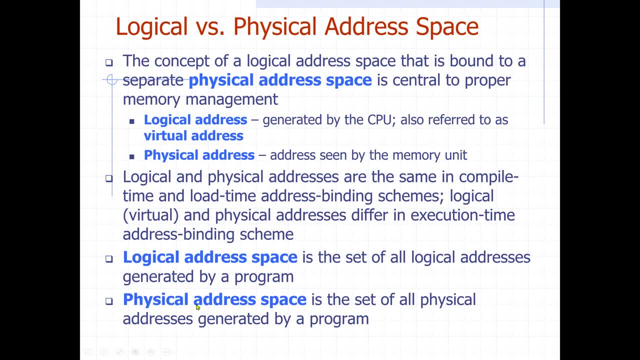 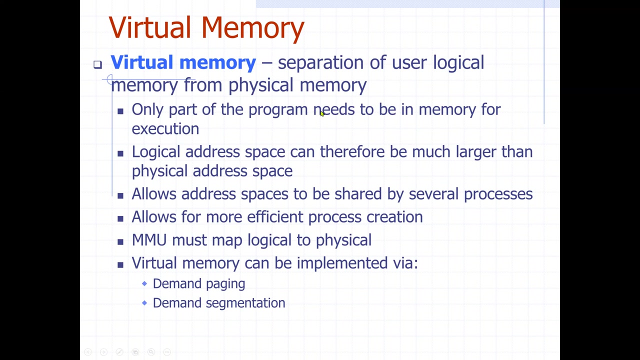 But during the execution time again they are different. So a logical address space is the set of all the logical addresses that was generated by a program, But the physical address space is the set of a physical address generated also by a program. So a ventral memory is the separation of a user logical memory from, again, physical memory. 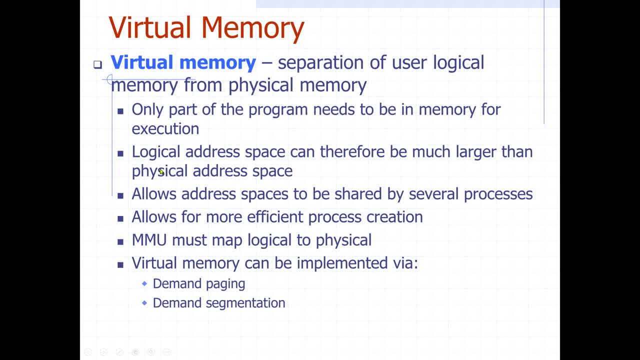 So logical- or logical address space can therefore be much larger than the physical address space and also only part of the program needs to be in memory for execution also. this allows address spaces to be shared by several processes. also allows for more efficient process creation and also the memory management units, which is mmu, must map the logical to physical. 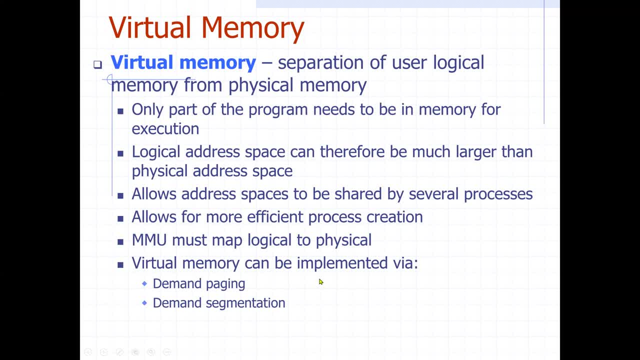 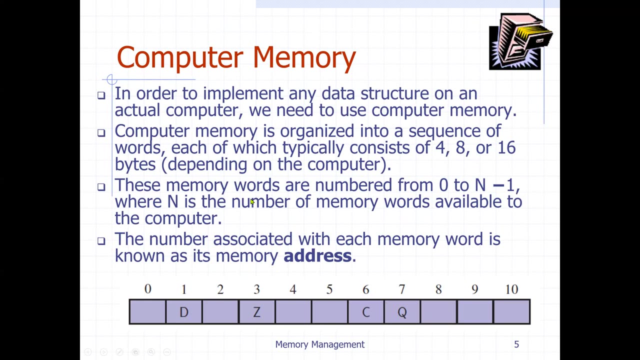 addresses. so virtual memory can be implemented through demand paging and also demand segmentation. again in this course we will not go details on the concepts here. the main reason why we are covering this section again: data structure. again, when we create any type of data structure it must be stored in a memory. so this topic normally 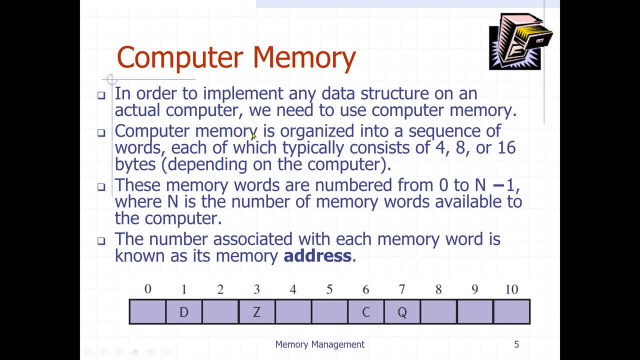 operating system is where we go. more details now with a demand paging. a page is brought into main memory only when a reference is made to a location on that page. now, if other elements of a memory management policy are good, the following should happen, which is when a process is first started. there will be a flurry of page faults as more and more pages. 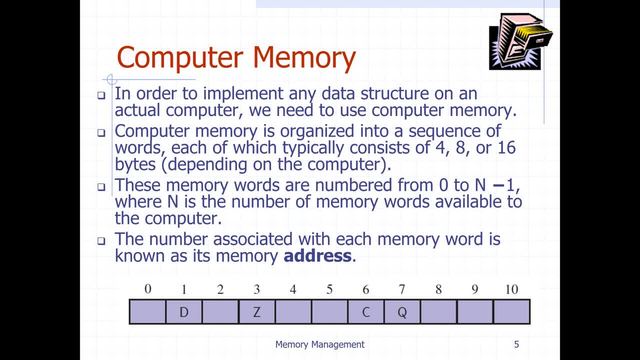 are brought in. the principles of locality suggest that most future references will be to pages that have recently been brought in. so after a time, matters should settle down and the number of pages fought should drop to a very low level, and we may discuss this more when we 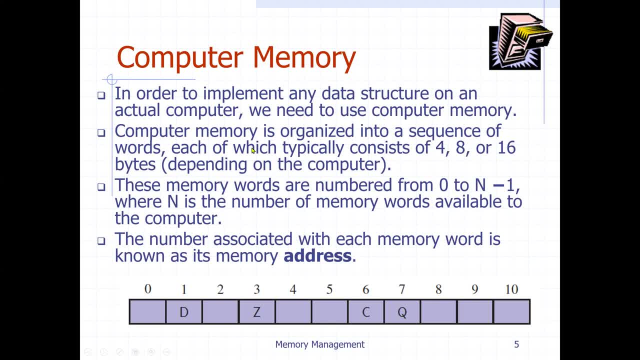 go further because some things might not go well, and drop them down the other side, then it is more efficient to bring in a number of contagious pages at one time rather than bringing them in one at a time over an extended period. Now, in order to implement any data structure on an actual computer, again, we need to use computer memory. 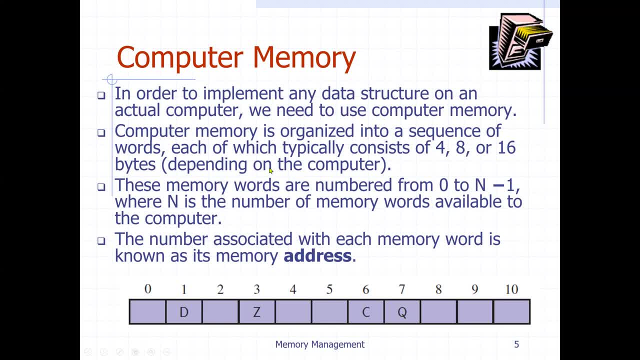 And this is the main reason why we are studying this chapter or this topic in our course- And again, this is the last chapter of our course textbook. So computer memory is organized into a sequence of words, each of which typically consists of 4,, 8, or 16 bytes, depending on the computer. 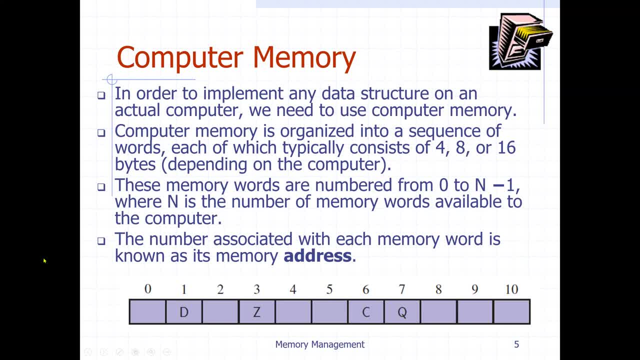 And again, these memory words are numbered from 0 to n-1.. Again, n is the size, where n is the number of memory words available to the computer. Also the number associated with each memory word. Every word is known as, again, the memory address. 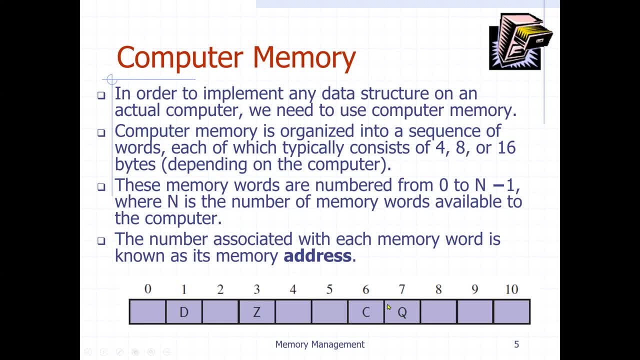 So we have an example here of a memory And we can see each box we call the cell has its own unique address And normally again when we are writing a program, we don't have to be more concerned where, for example, if we declare a variable or we create a data structure, where it should be located. 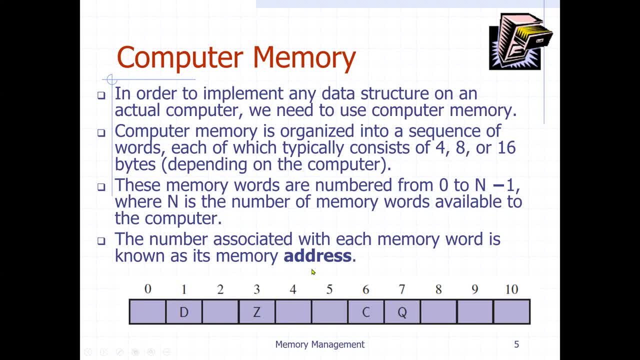 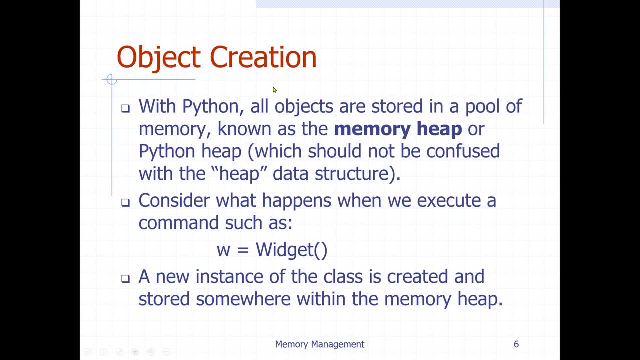 The operating system again, So we can randomly allocate the memory space for the process. So next is the object creation. Here we say, with Python all objects are stored in a pool of memory And this is known as the memory heap or the Python heap. 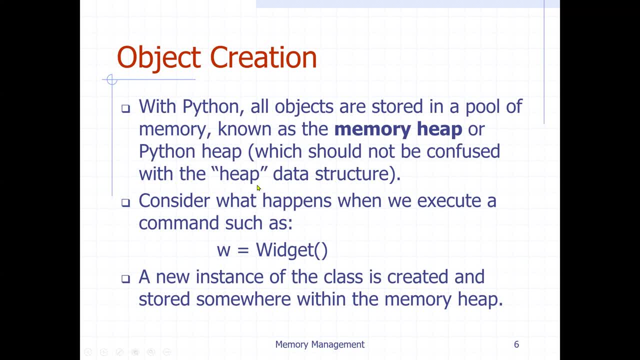 Now it's different from the heap data structure that we covered, So you have to say which should not be confused with the heap. This is the data structure. Now consider what happens when we execute a command, such as widget method or function assigned to W. 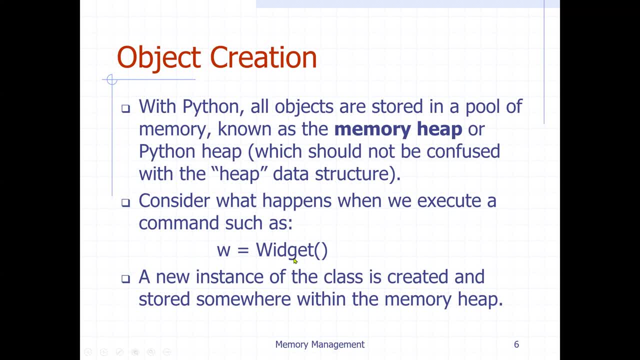 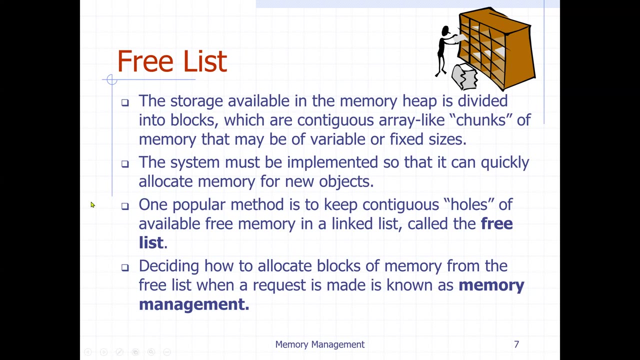 What will happen is that a new instance of the class is created and stored somewhere within the memory heap. Again, this process is done by the operating system. Next we talk about what is a free list. So a storage variable in the memory heap is normally divided into blocks, which are again a contagious area, like chunks of memory. that may be of a variable or it may be of a face size. 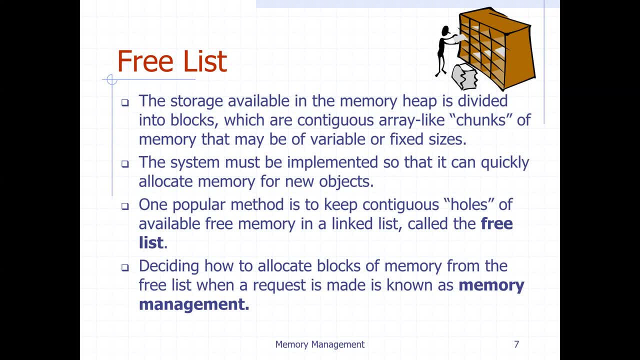 Now the system must be implemented so that it can quickly allocate memory for new objects, And one of the popular method is to keep contagious. So we have a free list of blocks, or also a variable free memory in a link list, And this link list is called a free list. 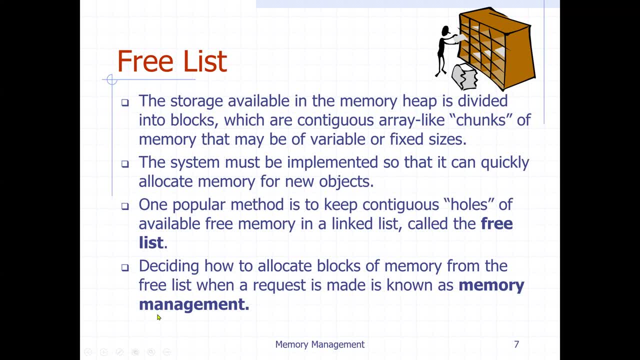 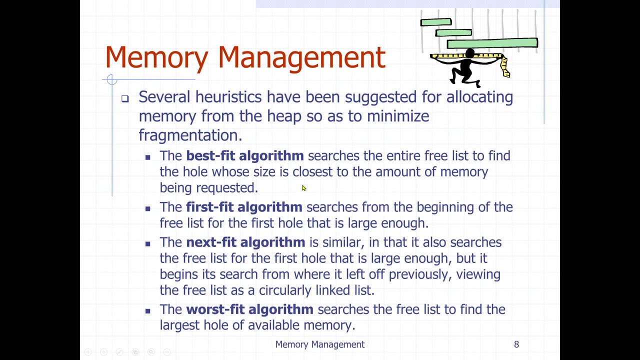 Now deciding how to allocate blocks of memory from a free list when a request is made is known as, again, memory management, And this is a very big topic in operating system. There are so many techniques we can use to manage our memory. 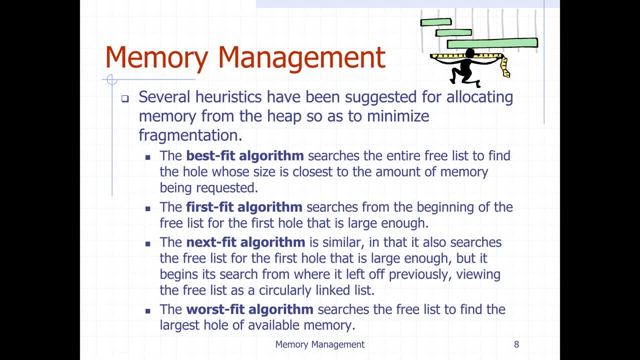 We can use memory management units again in our operating system, one of the pre-system functions. So several heuristics have been suggested for allocating memory from the heap And the goal is to minimize fragmentation. And these are some of the few algorithms. 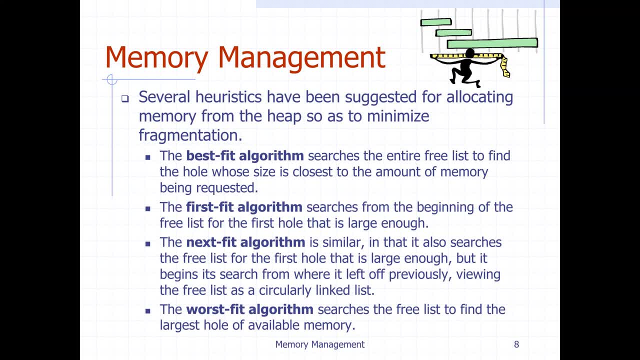 And again, these algorithms are discussed in many operating system tests. So, for example, we have the best fit algorithm And we also have the first fit algorithm, next fit algorithm and also the worst fit algorithm. So let's go through one at a time. 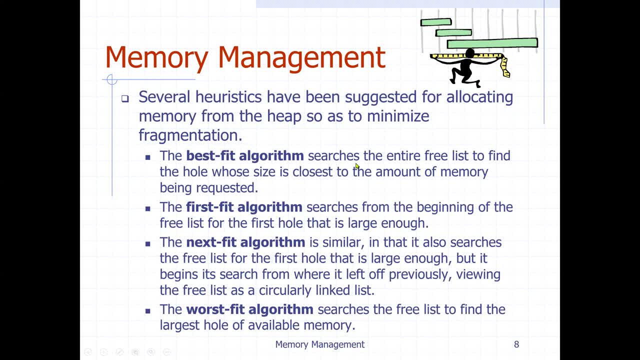 The best fit algorithm. normally we search the entire free list to find the hole whose size is closest to the amount of memory being requested. So if we find at least close to the amount of memory that we are requesting, then we use that And the goal. that's why it's called the best fit. 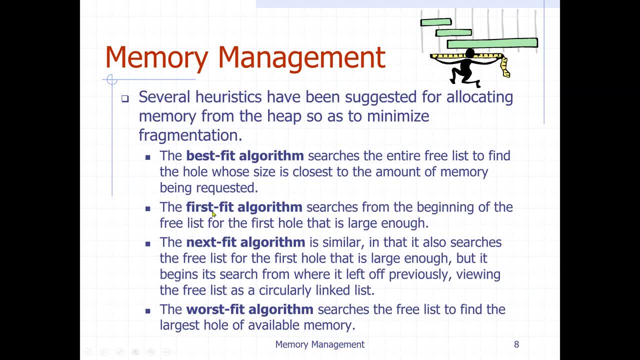 But the next one, which is the first fit algorithm. it searches from the beginning of the free list for the first hole that is large enough. So if the first hole is big enough to accommodate our process, Then it assigns The best fit. will go through all the lists to find the enough fit for our process, whether the same size or the closest. 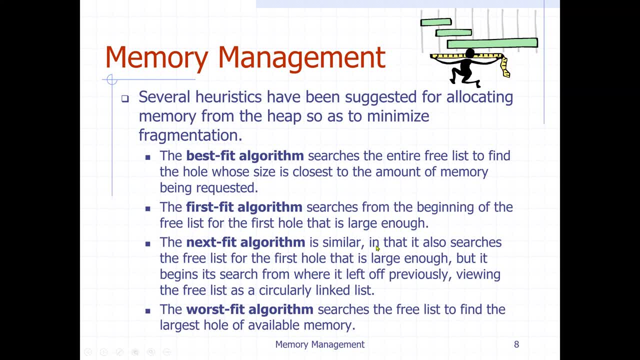 Now with the next fit algorithm is similar, But in that it also searches for the free list for the first hole. that is large enough, But it begins its search from where it left off previously, So that's why it's called the next fit. 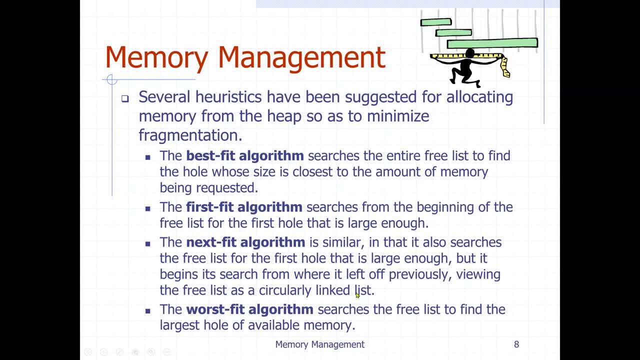 Viewing the free list as a circularly linked list, And the last one is the worst fit algorithm. This searches for the free list to find the largest hole of available memory, And next we have what we call the garbage collection. Again, this is a process of detection. 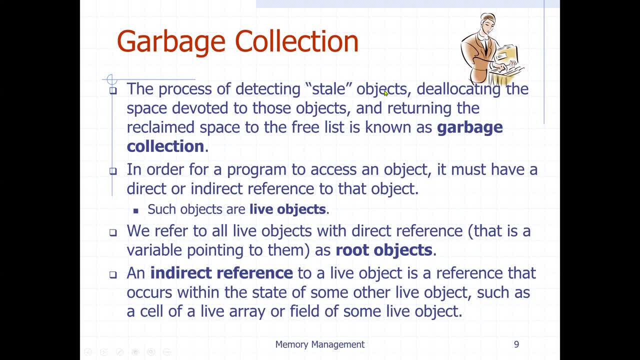 So we're collecting the store objects. For example in Java programming, if an object is the references or it's no more reference to any item, Again Java garbage collection method will automatically remove it or clean it. But we also have again a garbage collection tool in an operating system. 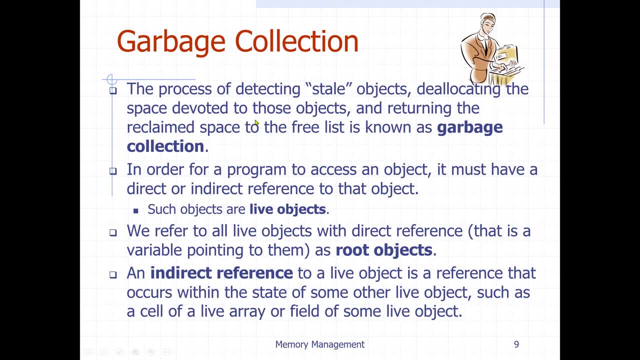 So, in the process of detecting the store object, they are locating the space devoted to those objects And then returning the reclaimed space to free list is known as garbage collection. This again is done by the operating system. Now, in order for a program to assess an object, it must have a direct or indirect reference to that object, such as objects, life objects. 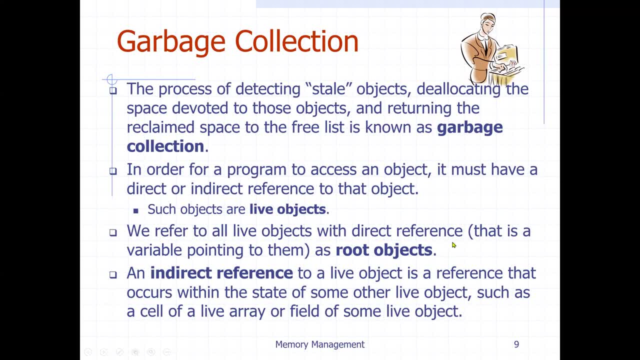 Also we refer to all the life objects with direct references- And that is a variable- pointing to them as the root objects. And also an indirect reference is to a life object. It's a reference that occurs within the state of some other life objects, such as a cell of a life array or a field of some life objects. 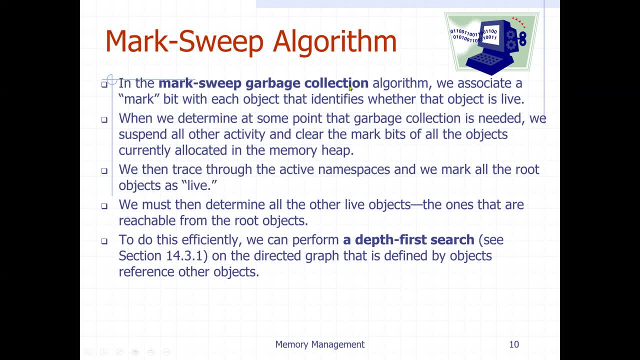 We also have what we call the MarkSweep algorithm. So with the MarkSweep garbage collection algorithm we again associate a Mark bit with each object that identify whether that object is life. Then when we determine at some point that that garbage collection is needed, we suspend all other activity and create a Mark bit of all the objects. 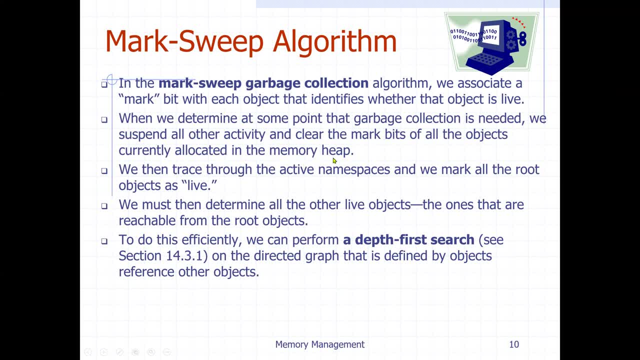 Now, when we then trace through the active namespaces, we mark all the root objects as life. Then we must then determine all the other life objects, the ones that are reachable from the root objects. Now, to do this efficiently, we can perform again the concept of depth-first search. 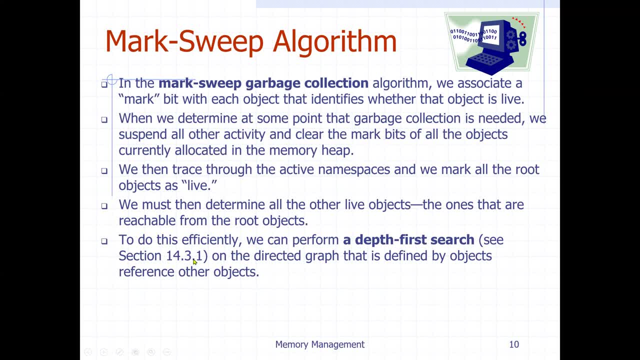 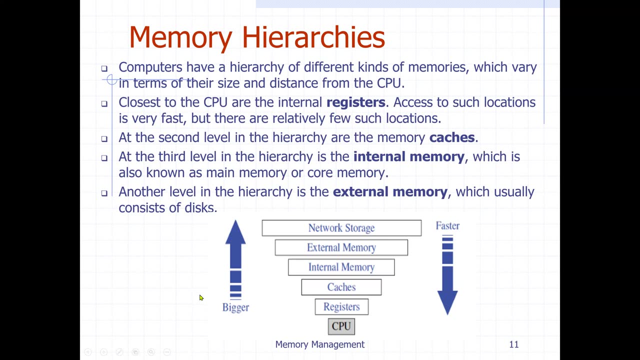 So we can define the depth of the page which we cover again in our Course Steps book, chapter 40, on a directed graph that is defined by object references or the objects. Now, one thing we should know also is the concept of a face-in, face-out policy. 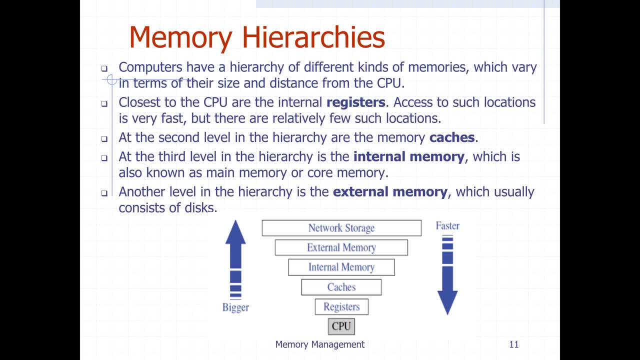 This normally would treat the page frames allocated to a process as also a circular buffer, And the pages are removed in a round-robin style. So face-in, again the face-out. So this is therefore one of the simplest page replacement policies to implement. 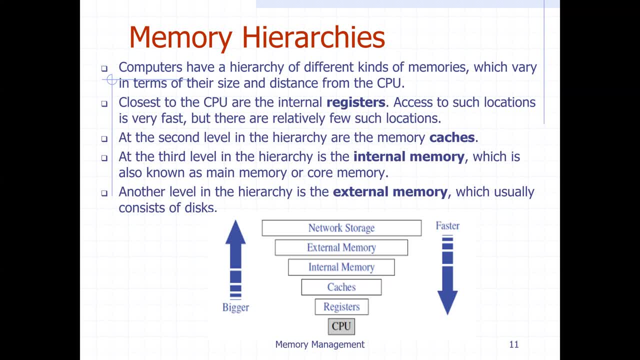 And the logic behind this choice, other than its simplicity, is that one is replacing the page that has been in memory the longest. Also, we have the memory hierarchies We know, from the lowest, which is the most expensive, to the largest. 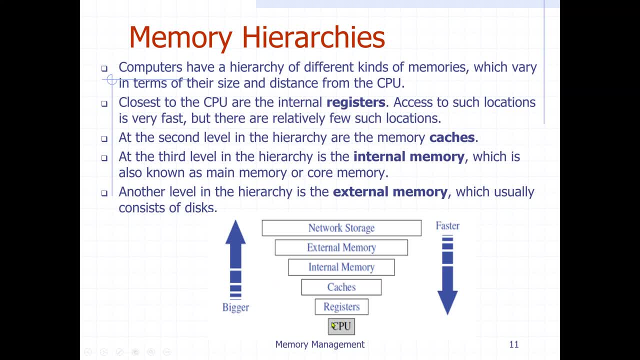 So normally the most expensive memory, which is very small, is the registers, And the closer the memory is to the CPU, the more expensive it is. So registers are normally inside CPU. Then we have the caches which are near to the CPU. 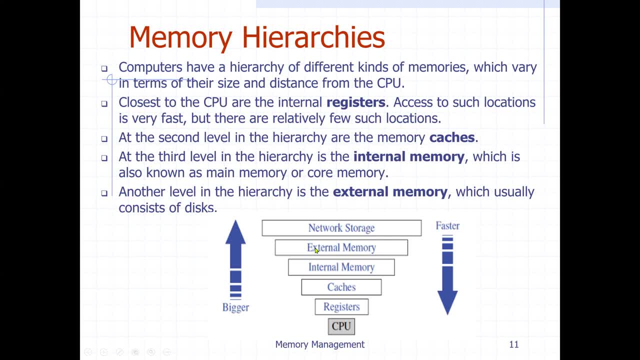 Then we have the internal memory, We may have external memory, then the network storage. So here we say, computers have a hierarchy of different kinds of memories which vary in terms of their size and distance from the CPU. So as the distance is shorter to the CPU, the faster the CPU can access the data from the memory. 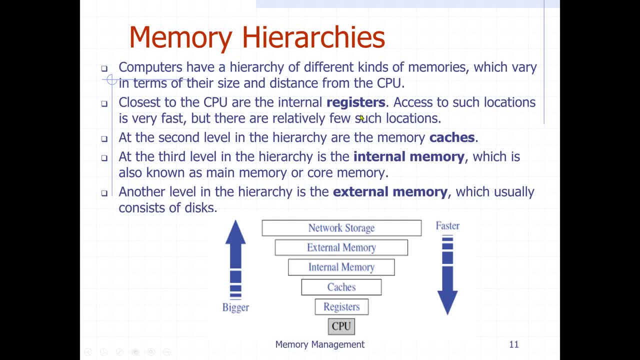 So here we say, the closest to the CPU are the internal memory, The closest to the CPU are the internal registers. Access to search location is very fast But there are relatively few search locations- Again, very expensive also. The second level will be the cache memory, which is very near to the CPU. 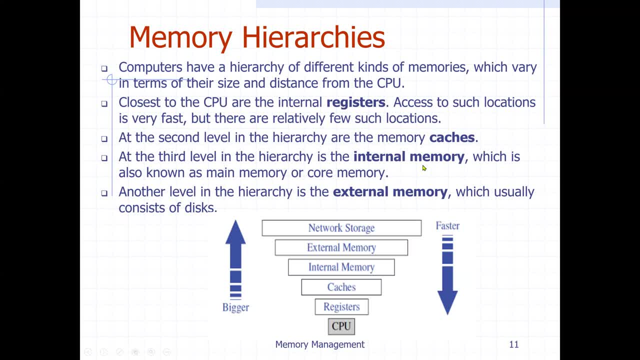 Then the third level will be the internal memory, which is also known as the main memory or the core memory. Then we may have the higher ranking, the standard memory, which consists of disk. So we can see, the bigger goes up, So registers is the smallest. 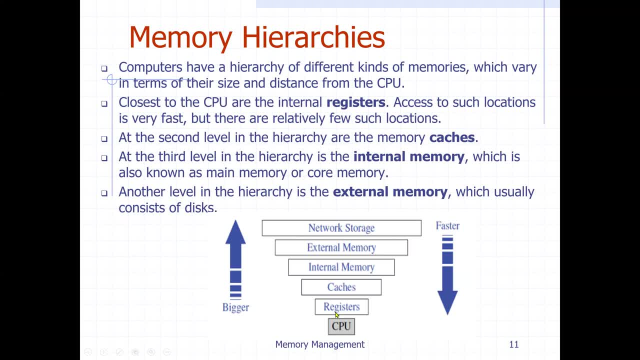 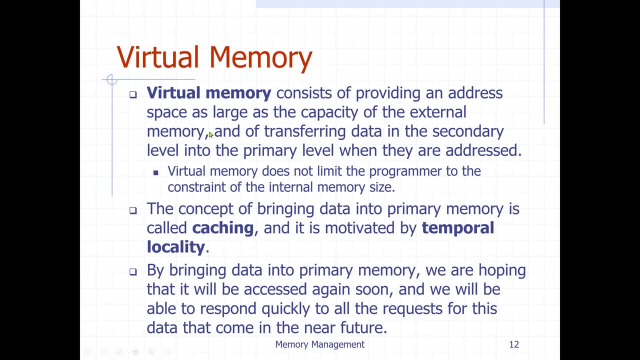 Network storage is the biggest. The fastest again is the registers. Then the most storage will be the network storage. So we said about the venture memory. Previously we said venture memory always consists of providing an address space as large as the capacity of the standard memory. 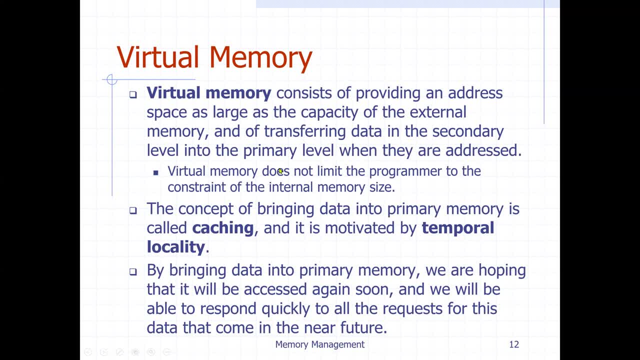 And of transferring data in the secondary level into the primary level when they are addressed. So normally, venture memory does not limit the programmer to a constraint of internal memory size. So the concept of bringing data into primary memory is called a caching And it's motivated by temporary locality. 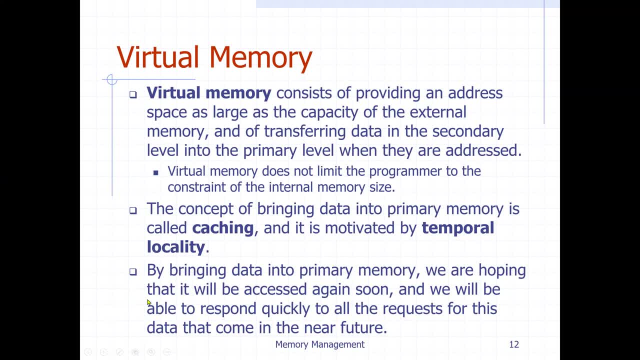 We also use the 10 principles of locality. So by bringing data into primary memory, we are hoping that it will be accessed again soon And we'll be able to respond quickly to all the requests for this data that come in in the near future. 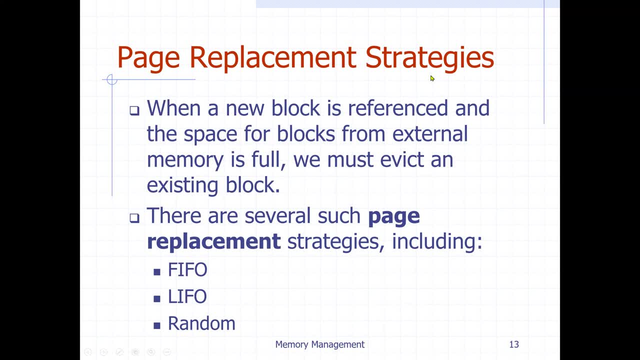 Then we have the concept of page replacement strategy. So we know that when the new block is referenced and the space for blocks from external memory is full, we must evict an existing block. So there are several search page replacement strategy, including the first in first out, or last in first out, or randomly. 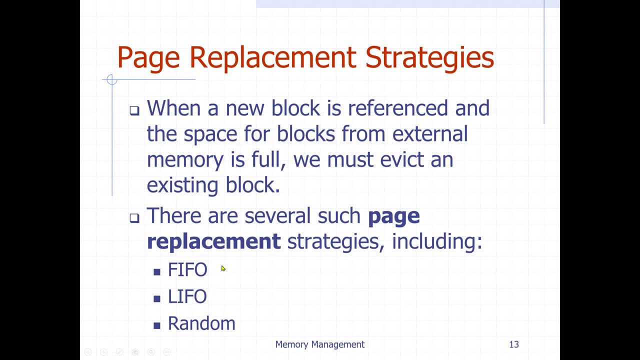 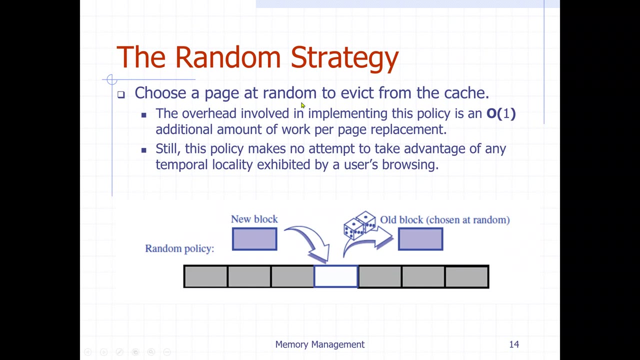 We also have the concept of least recently used policy. that replaces the page in memory that has not been referenced for a large, longest time. So here we have the random strategy. We choose a page at random to evict from the cache. So the overhead involved in implementing this policy is a big old one. 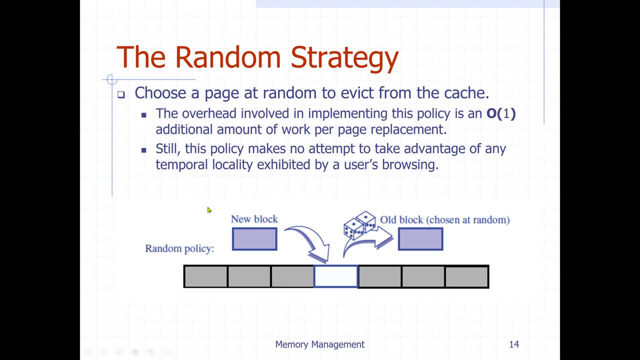 So additional amount of work per page replacement, But still this policy makes no attempt to take advantage of any temporal locality exhibited by the user browser. So we can see the random policy. A new block comes in, We replace it with the old block chosen. 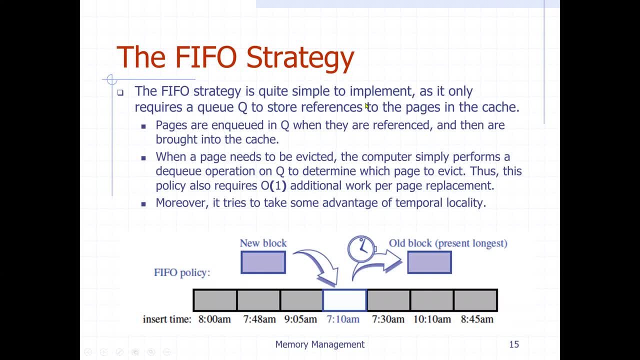 Now, with the first in, first out strategy is quite simple to implement As it only requires a queue to store references to the pages in the cache. So here we say the pages are in queue objects. So basically we insert the pages into a queue object when they are referenced and then are brought into the cache. 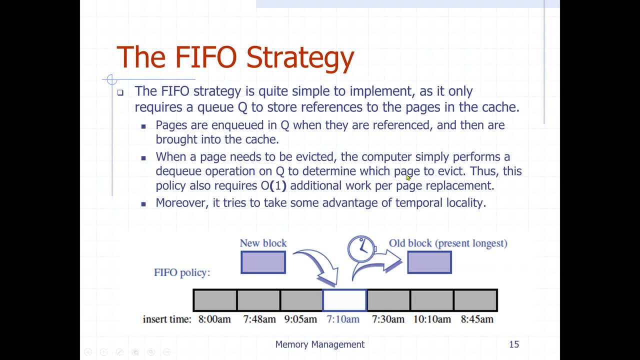 Now, when a page needs to be evicted, the computer simply performs a dequeue operation. So first in, first out on the queue object to determine which page to evict. So we say this policy also requires a big old one. Additional work per page replacement. 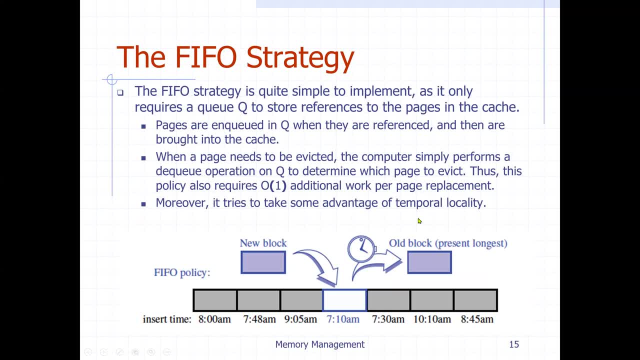 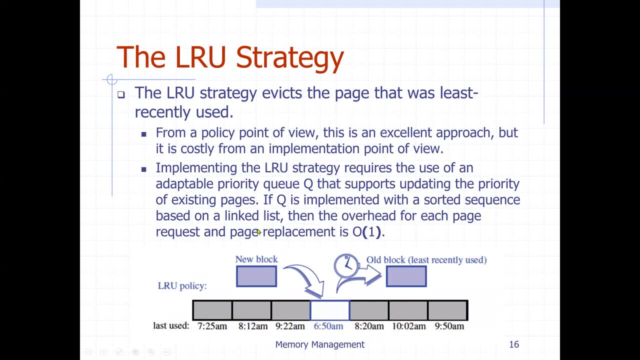 Moreover, it tries to take some advantage of temporal locality. So, again, this policy is very simple. The whole concept again is using a queue or circular queue concept. Now, with the least recently used policy, it replaces the page in memory that has not been referenced for the longest time. 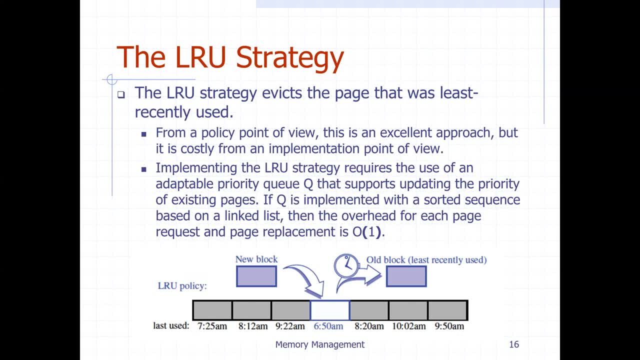 So, again, as we said earlier, by the principles of locality or temporal locality, this should be the page least likely to be referenced in the near future And also, in fact, the least recently used policy does nearly as well as optimal policy. 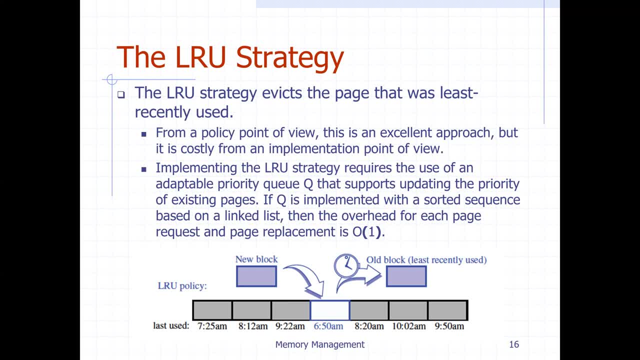 But the problem with this approach is the difficulty in implementation. So again, difficult implementation. One approach would be to tag each page with the time of its last reference, And this will have to be done at each memory reference When each memory reference both instruction and data. 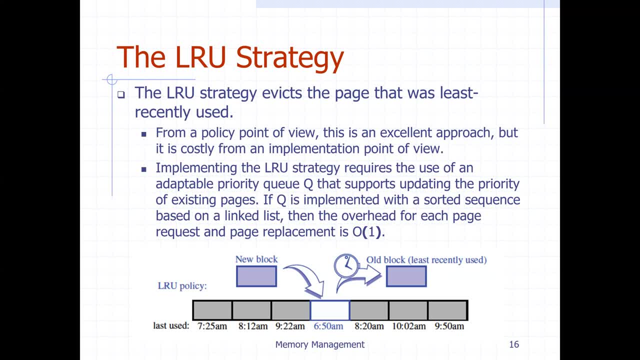 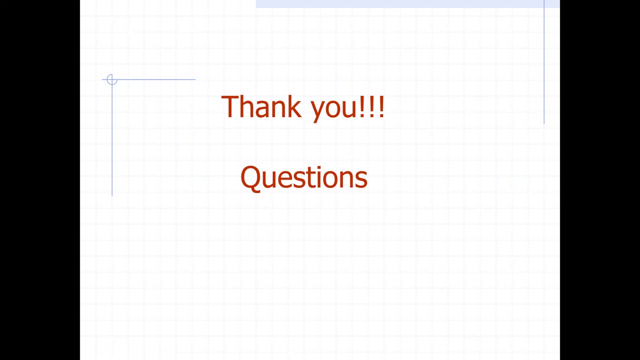 And also if the hardware will support such scheme, the overhead will be tremendous. Also, it has a big old one overhead. So again, that will be the conclusion of our lectures on Chapter 15-1.. And we will go to the next lectures, which will be 15-2.. So again thank you.